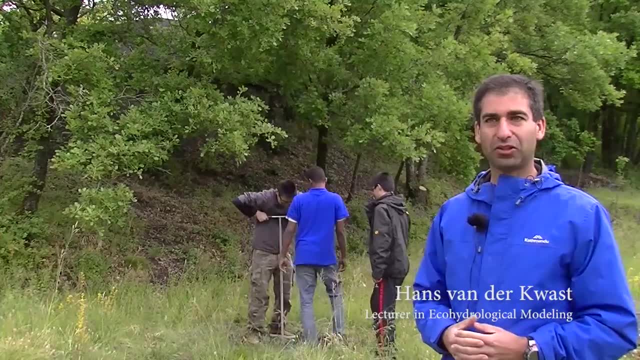 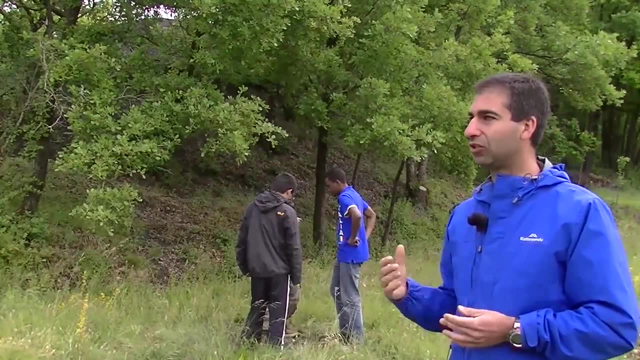 So I think from an educational point of view it's a very important step that people go to the field and measure, Because behind your computer and from the books, all the theory, it's all nice, But these students now learn that there's a big difference between theory and practice. 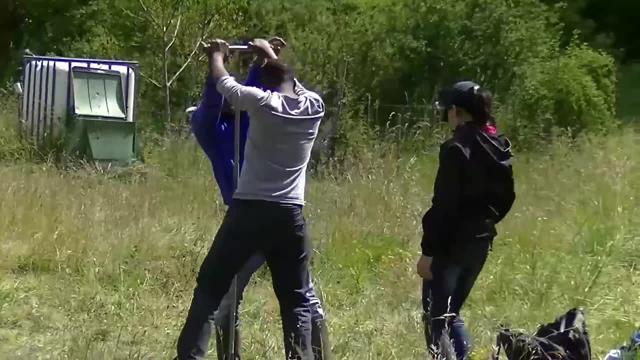 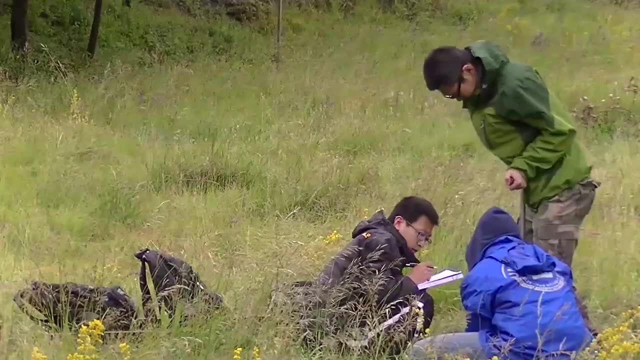 You have to be here in the field and see that things are not so perfect. You can drill a hole into a stone and then you have to start over again. And in the future, when in their jobs- it's very important When they send out people to the field that they really know- remember this feeling of being in the field. 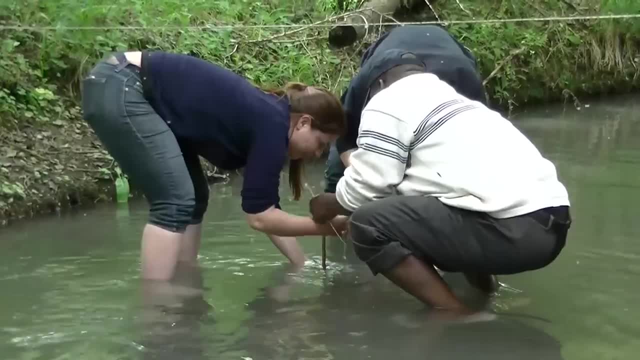 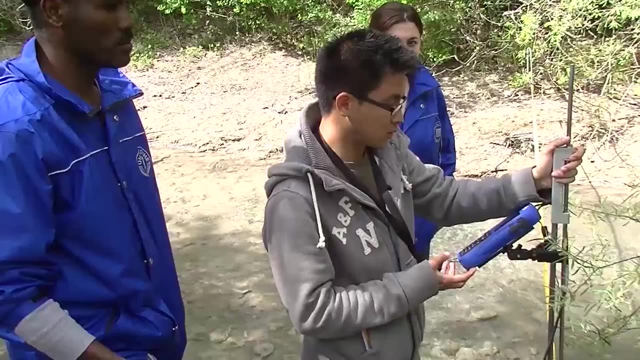 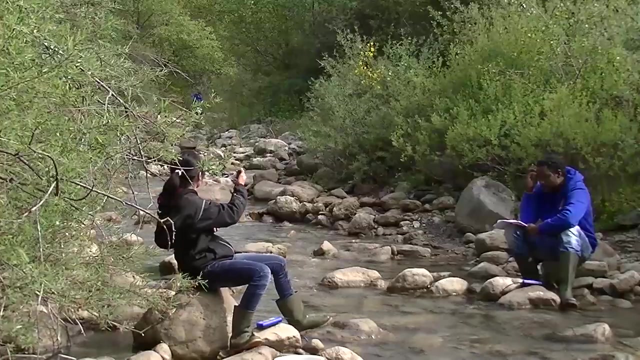 Later, when they use data in models, for example, or for evaluating how much water there is in the river, they have some feeling about well, how accurate is that data? But they can value it because they now understand what it means to actually capture discharge data. 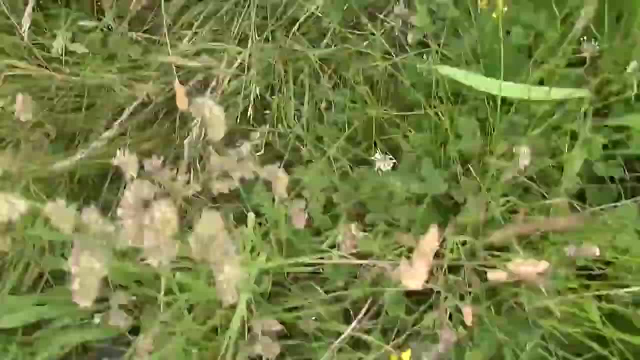 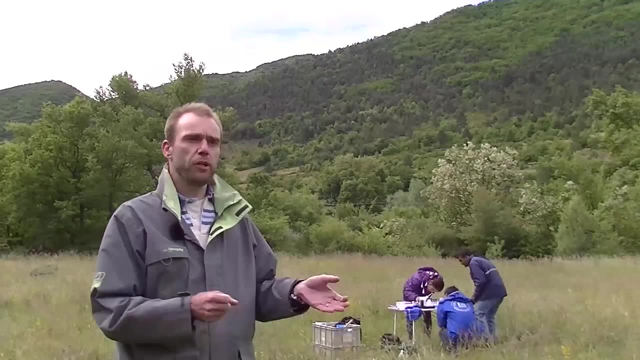 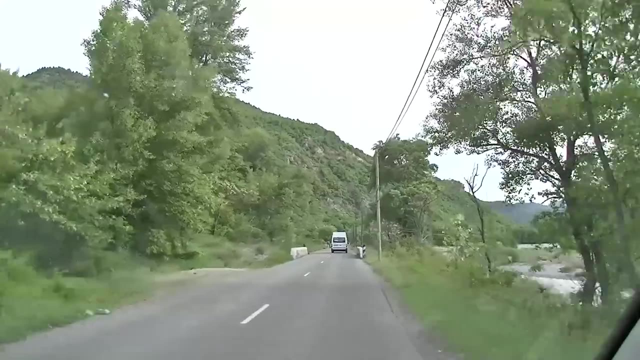 And then they go into the field with their assignments- different assignments- And for the hydrology and water resource students this is getting to know the time-dependent water balance of a catchment And what are the factors that influence that water balance. Also, land use is a very important aspect there. 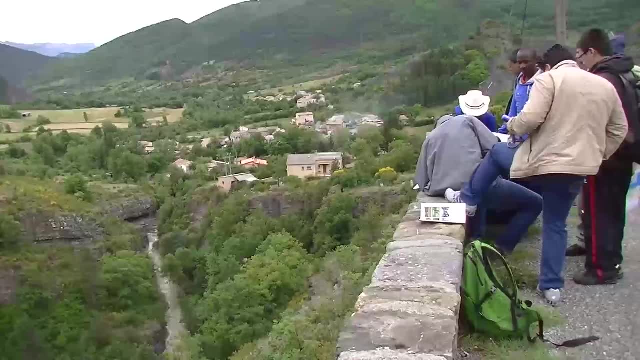 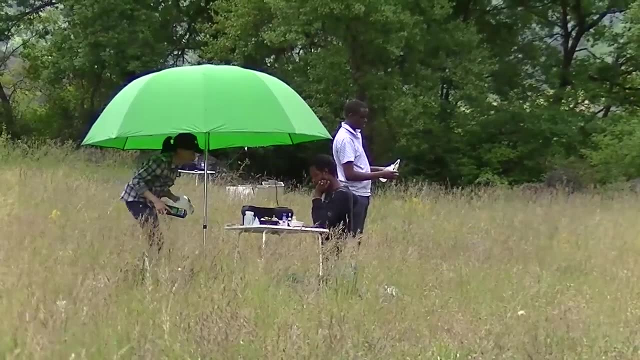 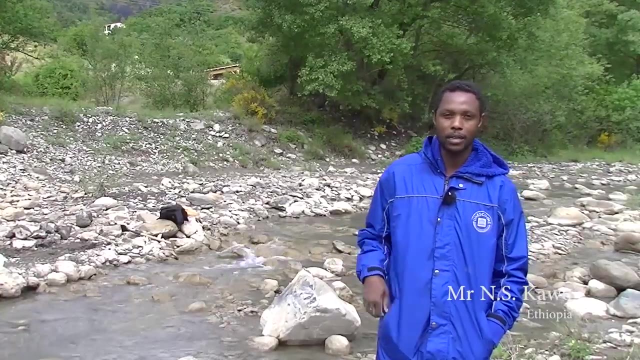 So if you have human activities that are over everywhere around us, how they affect both the hydrological system in terms of quantity as well as quality, how they affect the quality of the water- Yesterday also, we did water quality analysis. We identified water type. 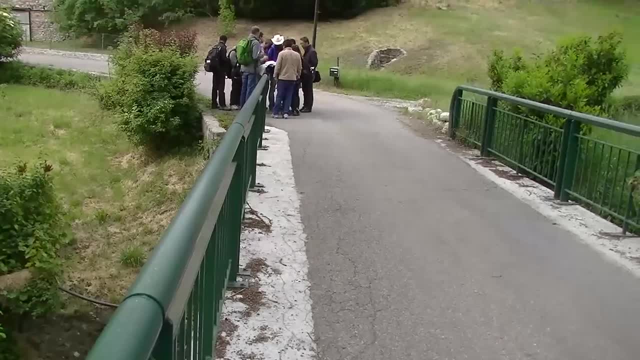 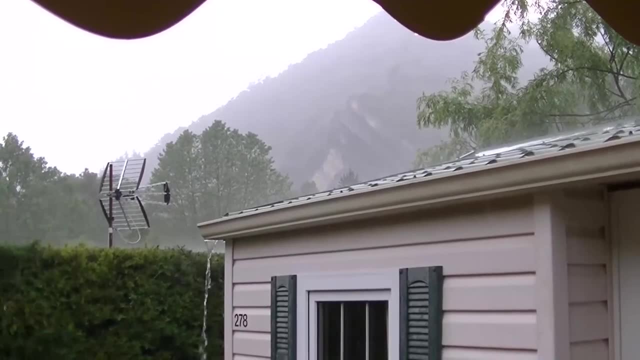 We are getting a lot of experience. This is important to know what happens, for example, if there's a rainfall event, How quickly will the water end up in the river and do we have to take measures? But also, on the longer term, what if? scenarios? 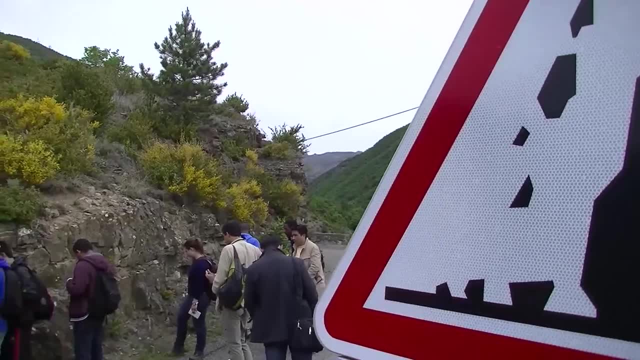 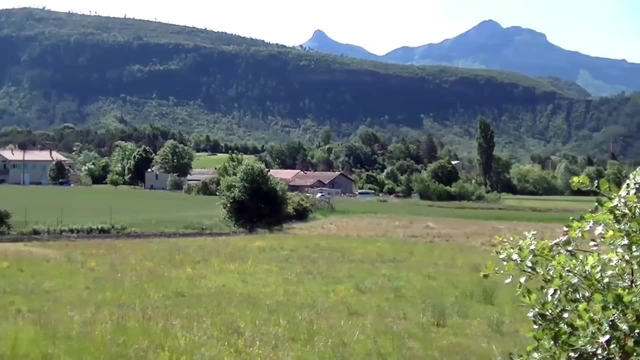 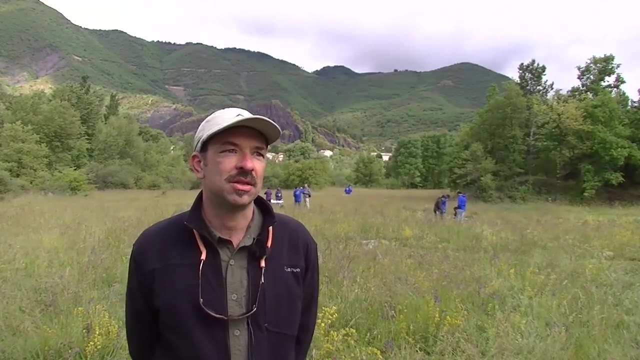 What if the climate changes and more rainfall, or the rainfall will be more intense? What will happen? What will happen in that catchment? The river basin development participants design a sediment protection structure like a check dam, So to avoid sediment to come downstream and be sedimented nearby the villages.